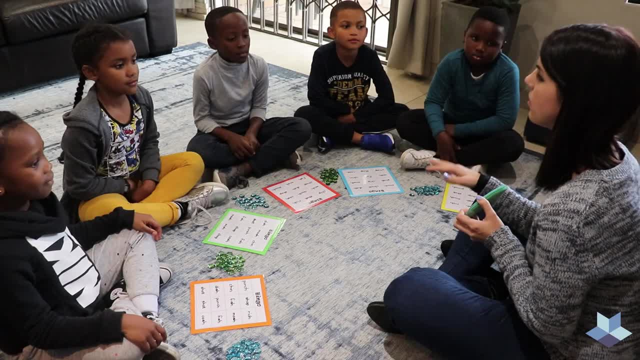 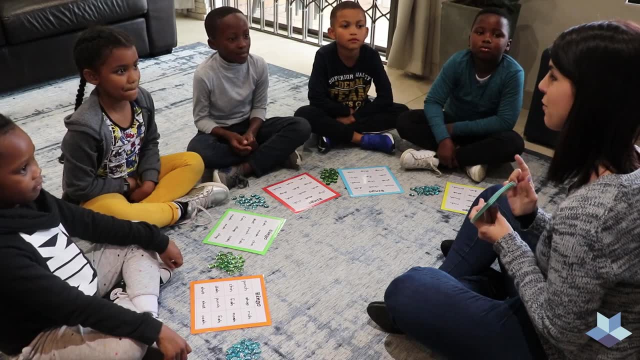 to read the word and then you need to look if the word is on your board. If the word is on your board, then you can put a counter on it. Some of you might have two of the same words, so you need to look here. 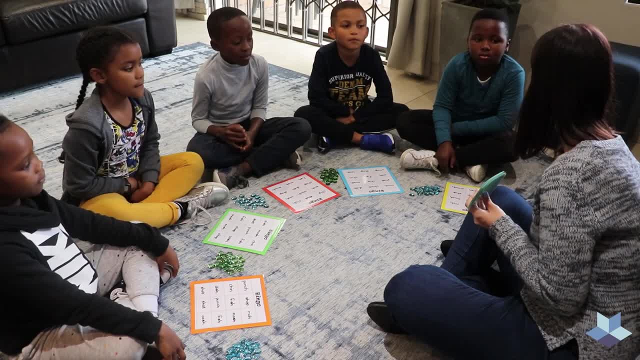 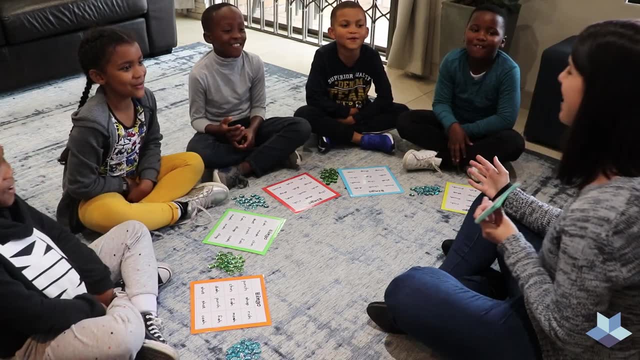 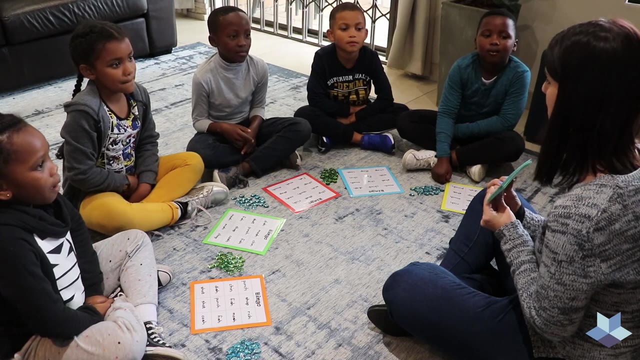 Then you need to get four words down and if you do, do you know what? you're going to shout Bingo, Bingo, And then you are the winner. Okay, should we try First word? we're going to sign out first, remember So: M-A-C-H, M-A-C-H- Look for the word. Okay, next one: M-A-C-H. 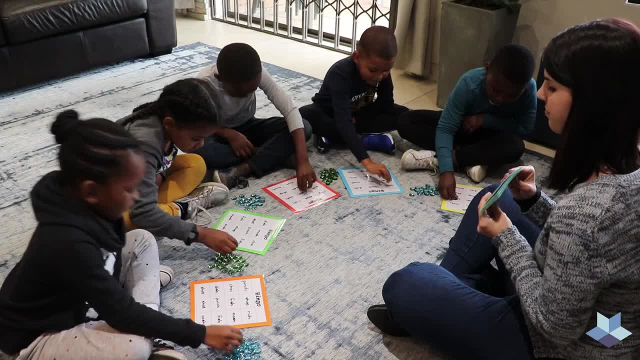 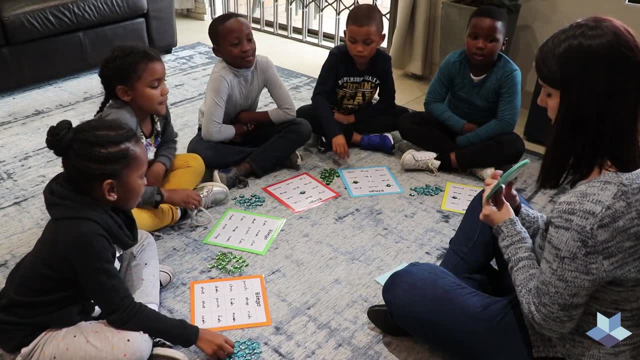 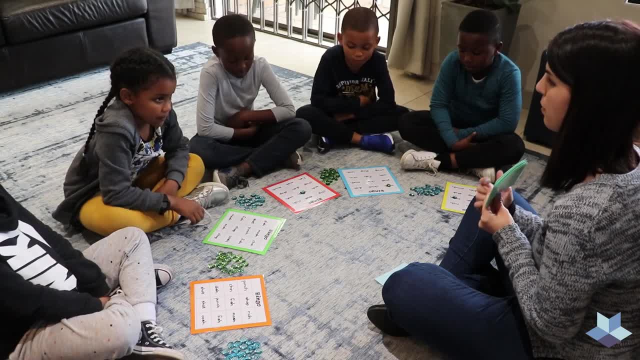 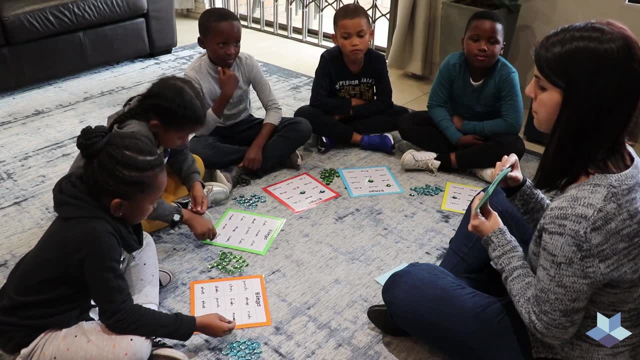